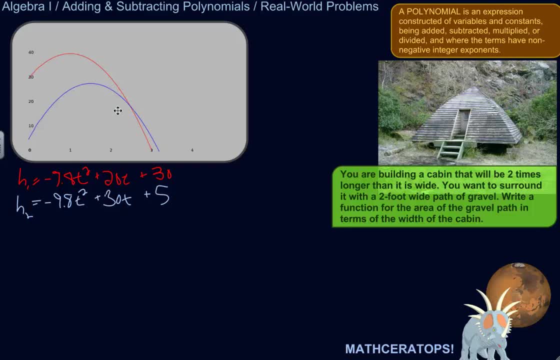 Alright. so when would you ever need to add or subtract two polynomial expressions in real life? It depends on what you mean by real life. I take that to mean you're trying to describe an actual situation mathematically and you need to solve a problem based in reality. 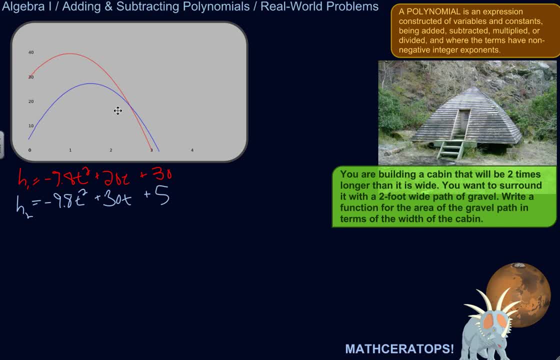 mathematically So, for example, meaning it's not just numbers, that the numbers mean something. So there's a couple of examples I thought of in which you would need this skill, or you could approach them from this perspective, And I'll let you understand these. 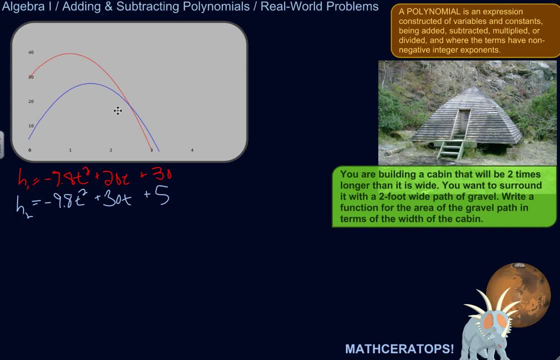 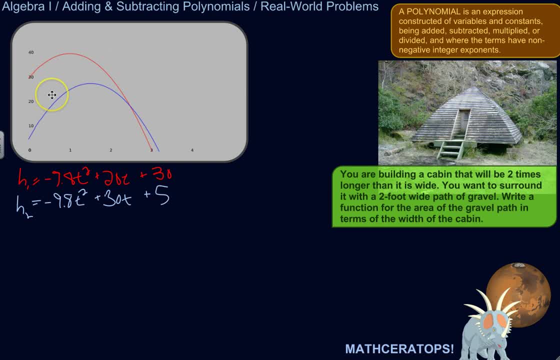 trying to solve a problem based on real life. And you're trying to solve a problem based on real life. And you're trying to solve a problem based on real life And you are shooting things into the air. you know like you do. Let's say pumpkins, No, let's say rockets, two rockets. 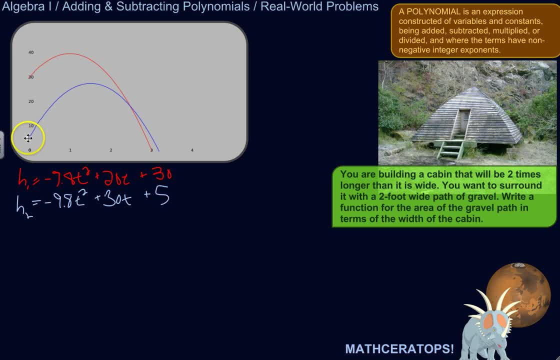 in the air. So one of them, you're starting pretty low to the ground but with a lot of force, so it has a higher initial velocity. And one of the rockets you're shooting you're starting off higher up in the air, like maybe on a hill or something, And you're starting. 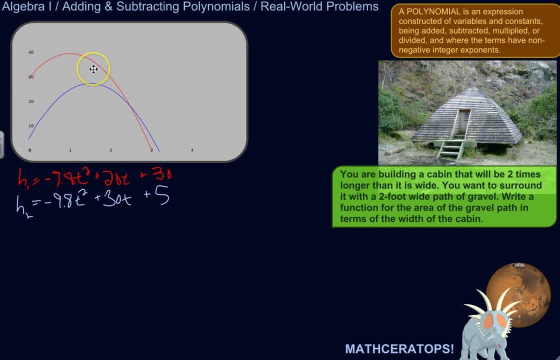 but with less force, And you're interested in knowing how far apart vertically the two things are if you shoot them at the same time. You want to write an equation that tells you, at any given point in time, how far apart vertically are these two projectiles. 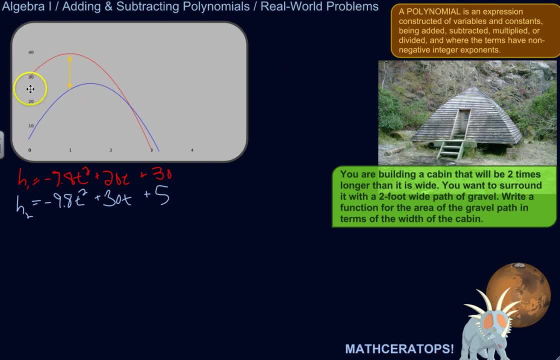 Okay, So here's the graph of the two projectiles. So here is the height above the ground. So 10 meters, 20 meters, 30 meters, 40 meters. Maybe I should label those meters, Let's see. And then this is time in seconds. 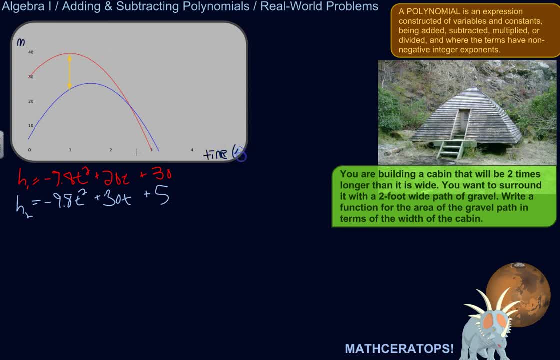 Tim, Not Tim. It's time Time in seconds. So here's where we start. You know, after one second, here's where they are. After two seconds, here, Here's where they are, Three seconds, et cetera. 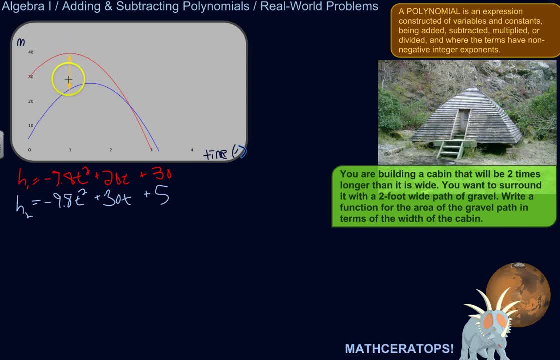 All right. So say you want to write an equation that tells you how far apart they are vertically, Because maybe you want to find out when do they crash into each other, Like you're really interested in knowing this. Well, in order to know that, 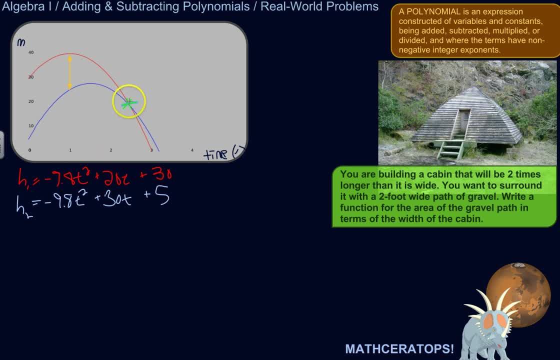 maybe you want to write an equation that tells you when that happens, You know? in other words, if you write an equation that shows the distance between the two projectiles, you can solve it for when it is equal to zero, meaning the distance between them is zero. 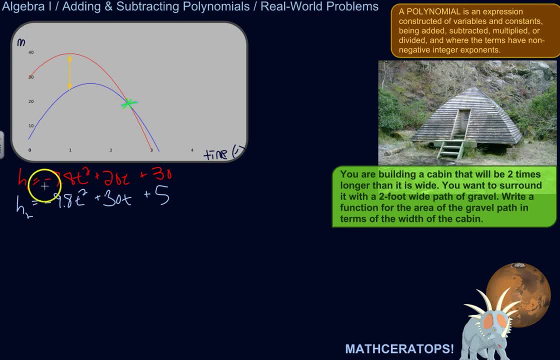 ie they've just smashed into each other, Right, All right. So that's the exercise here. So the equation for this first guy is negative: 9.8 times t squared plus 20t plus 30.. And that's your general equation for, or that form of an equation is for, the distance above the ground. 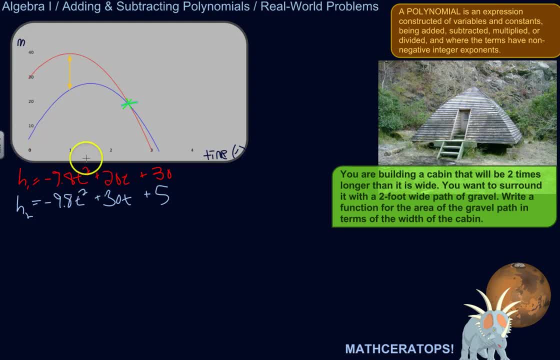 when you're shooting something off the surface. This part of it is the acceleration due to gravity. This part is saying what your initial velocity is. So this means 20 meters per second. So we're shooting this guy at 20 meters per second. 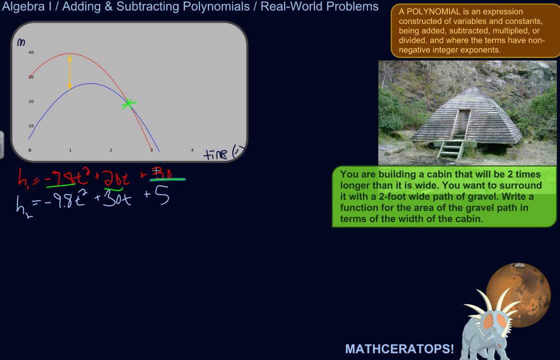 And this is how high above the ground you start. Right, Okay, So, and then the second one is: you know, acceleration due to gravity is the same. This is both. we're both on planet Earth. The initial velocity is 30 meters per second. 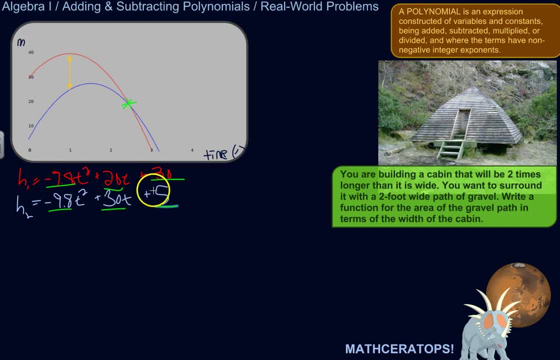 And the initial height is 5 meters. All right, So this guy is starting lower down, but we're shooting him at a higher velocity And we want to see, kind of when they catch up, Basically when. yeah, we want to see. we're going to pretend. 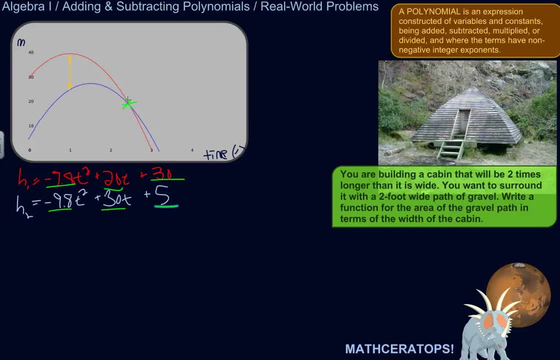 that we can shoot them directly on top of each other. Well, I don't know. We basically want to find out when, vertically, they are. the distance between them is zero. Okay, I don't know, Maybe this is a contrived situation, but work with me here. 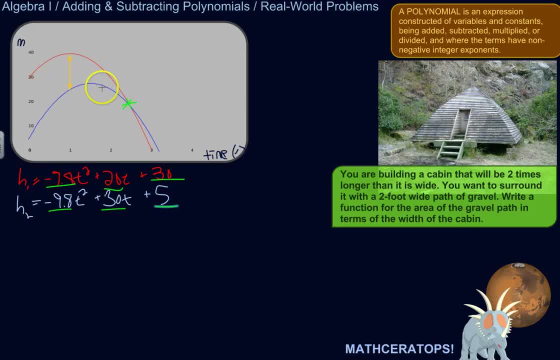 All right. So what we can do is: so we've got an equation for this and we've got an equation for this. Well, what's the difference? distance between them? We just subtract this from this, Right, If I've got something that's this tall and I've got something that's this tall. 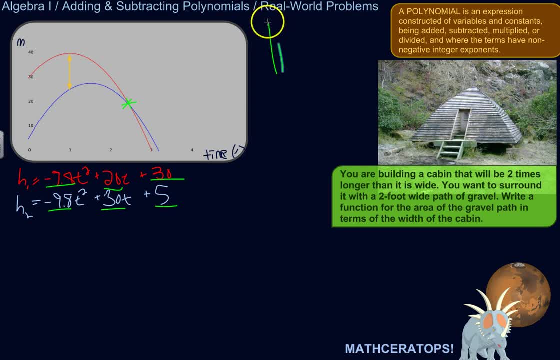 and I want to know what the difference between them is. I take you know, let's say that's 10 meters and that's 4 meters. Well, this is 6 meters. therefore, right, This is just slightly more complicated because this is you know. 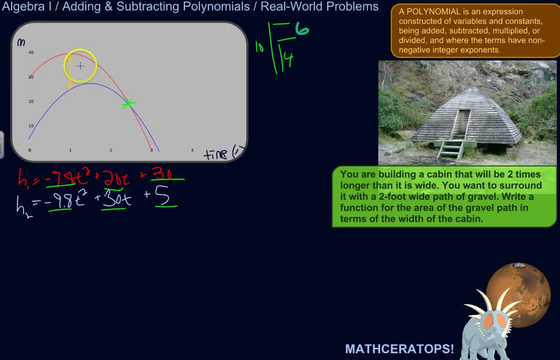 an equation that describes this. It's not just a number. Okay, So I'm going to subtract this from this, and that will give us the equation that tells us how far apart vertically these two projectiles are. So I'm going to subtract. Okay, So I'm going to subtract this from this, and that will give us these equations. 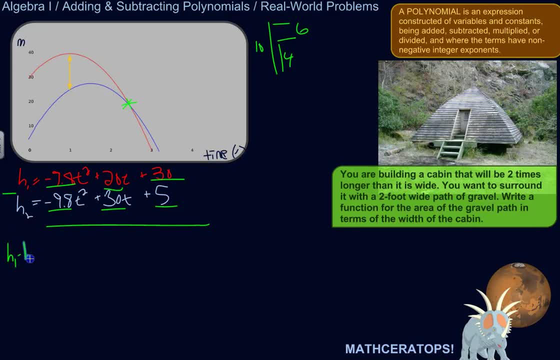 So we've got so h1 minus h2, so ie the distance between them is okay. so negative 9.8t squared minus negative 9.8t squared. So minus a negative would actually mean you're adding that. 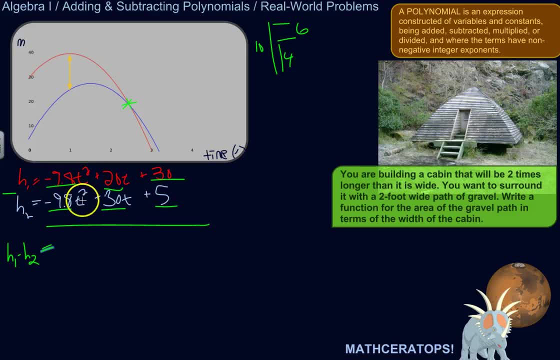 So you're taking the negative something and adding the positive of it, so this term it just cancels out. so that's nice. And then we've got 20t. minus 30t would be negative 10t. So you add or subtract like terms. 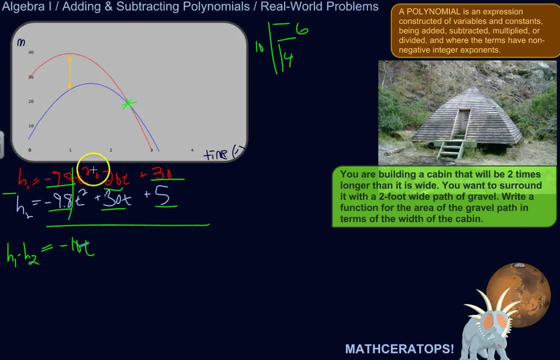 So these are like terms because they're. they both include t squared. These are like terms because they include just t, And these are like terms because they're both constants. Okay, So 30 minus 5 is 25.. Yeah, So this would be our equation that tells us for: 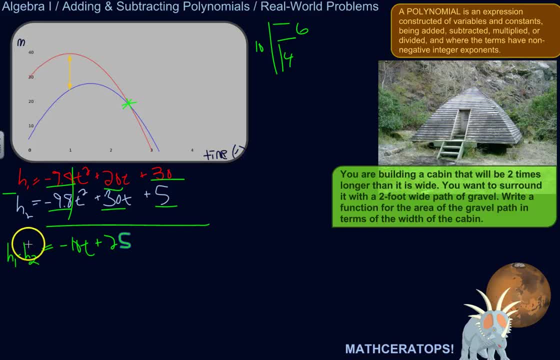 for a given time, how far apart these two curves are from one another. Yeah, All right, So we could solve that, So we could, so we could say: all right, we want the distance to be zero, Let's solve for when the distance is zero. 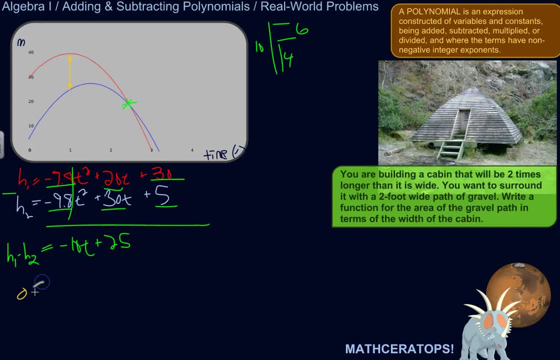 So we could say zero switch colors to indicate that I'm doing something cool. Zero equals negative 10t plus 25.. Okay, I just want to get t by itself minus 25, minus 25.. So negative 25 is equal to negative 10t. 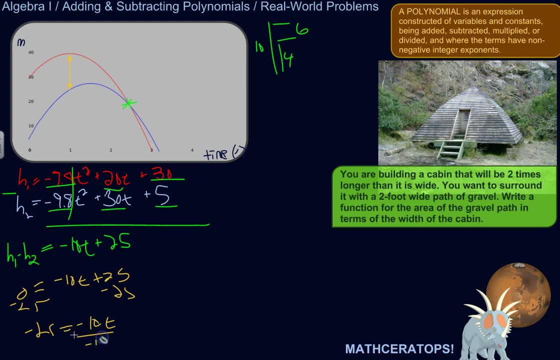 Okay, Divide both sides by negative 10,. divide by negative 10.. So negative 25 divided by negative 10 is what is that? Two and a half, yeah, 2.5 seconds. So after two and a half seconds these projectiles are at equal heights. the different 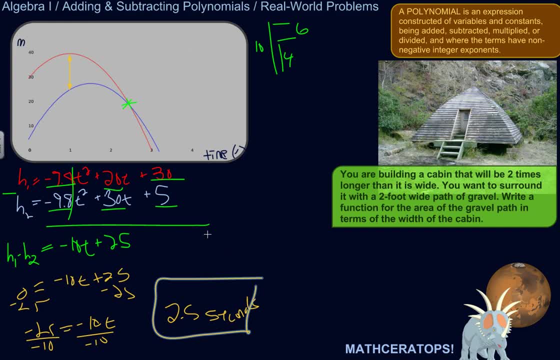 the distance between them, Yeah, Is zero. All right, Kind of see where we're going with that. All right, Let's look at this second example. Suppose you are building a cabin that will be two times longer than it is wide. 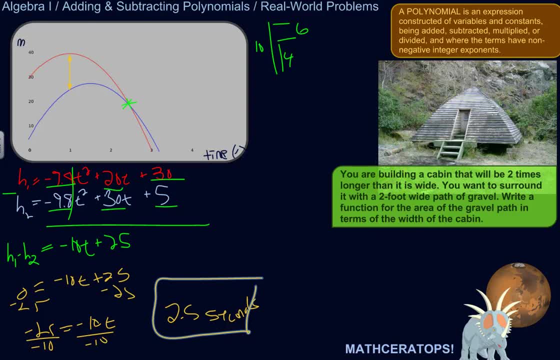 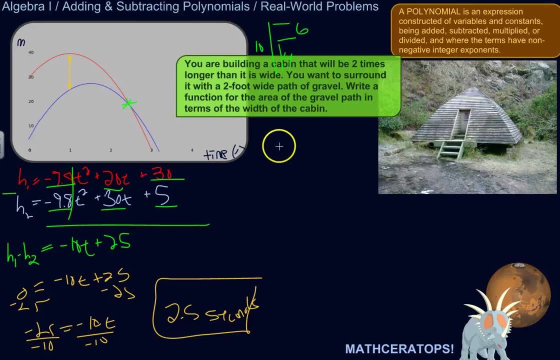 So I'm going to start. I'm going to draw a diagram here. Let's move this up here. Okay, All right. So I want to build a cabin that's two times longer than it's wide. Let's make it brown. 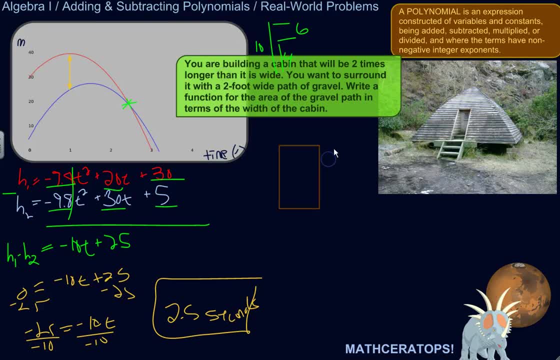 Because it's a cabin, You want to surround it with a two-foot-wide path of gravel, right, you know, maybe to catch the rain runoff or something like that. Write a function for the area of the gravel path in terms of the width of the cabin. 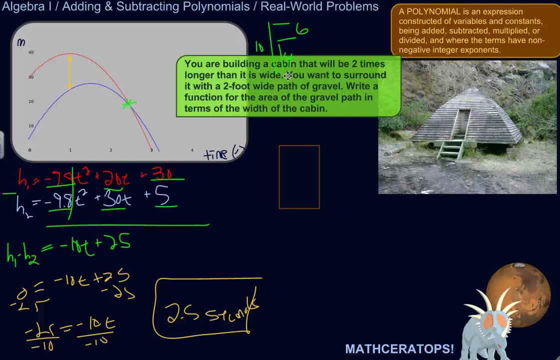 So maybe you want to figure out the area of the gravel path because you're maybe you've got some gravel available and you want to figure out: well, if I design the cabin this way, will, would I have enough gravel to you know. 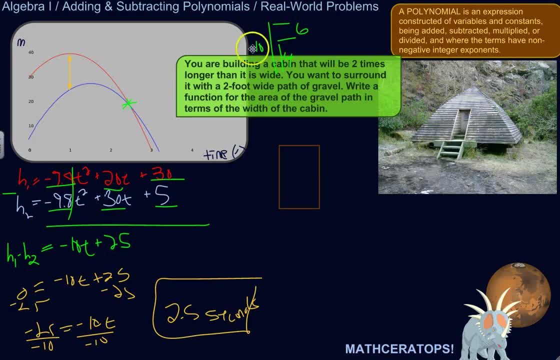 surround it with a two-foot path, or am I going to have to adjust that? All right, So I want a cabin that's two times longer than it is wide, because it looks nice that way. Okay, I mean, you know, I'm kind of simplifying things for the sake of this example. 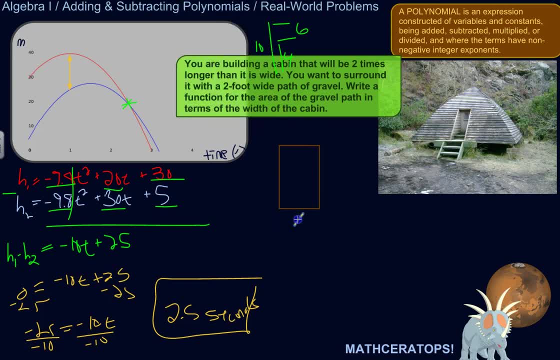 So we don't know how wide or how long it's going to be, but but if it's X feet wide, it'll be 2X Feet long, And actually let's just put that inside there, because I want to draw the the gravel. 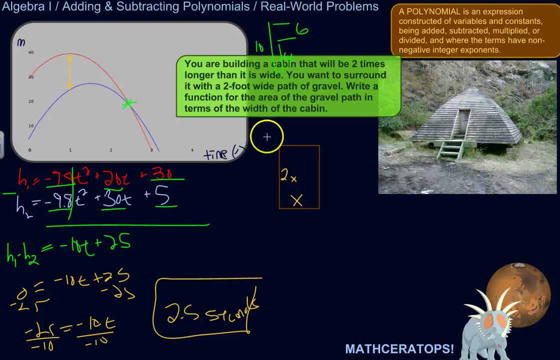 Now, we want a gravel path. Let's make that gray. Okay, We want a gravel path. Let me make that bigger, so it's easier. Is this interesting to you? I hope so. Okay, I feel like I ramble a lot, but hopefully this is making sense. 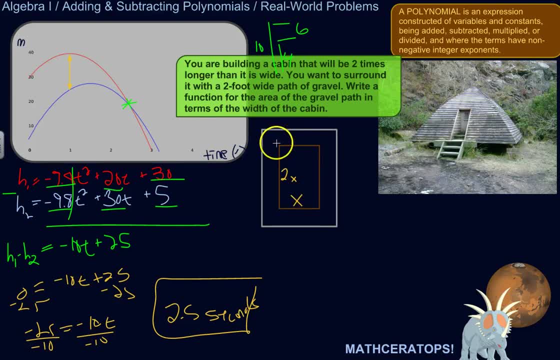 Okay, So my cabin is going to be X by 2X feet. The gravel path is going to be, it's going to be. I'm going to add two feet, You know, to both right in, in every direction, so it's two feet around. 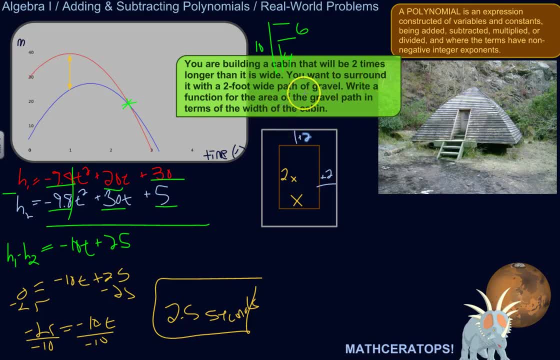 Okay, So I want to. I want to function for the area of the gravel path. So I want- really I want- the area of this outside piece. So, if you look at it, what I really want is what I. what I can do is if I write something that describes the area of the big rectangle. 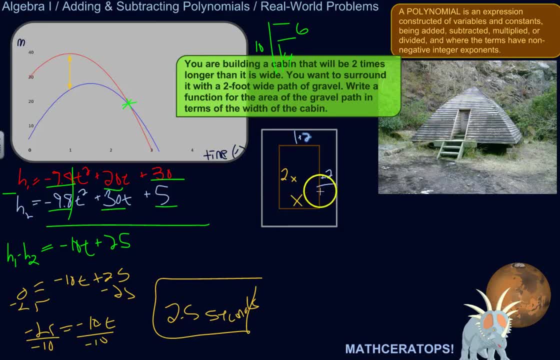 Okay, and I subtract the area of the small rectangle, the cabin- all I'm left with is the area of the gravel, Right In fact, yeah, Right. So big rectangle minus small rectangle means you're just left with that difference, right? 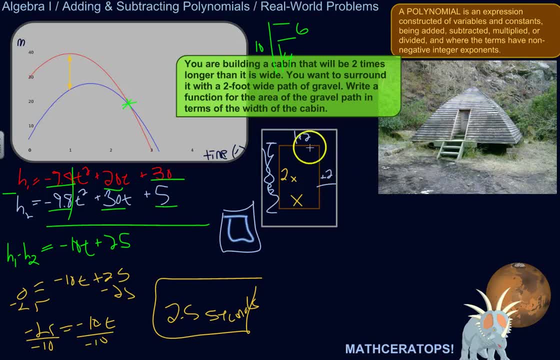 So let's write an equation for the area of the Okay, of the big rectangle, and then let's write one for the area of the smaller rectangle, and then we'll subtract them, Ding, ding, ding, And then we'll have our equation. 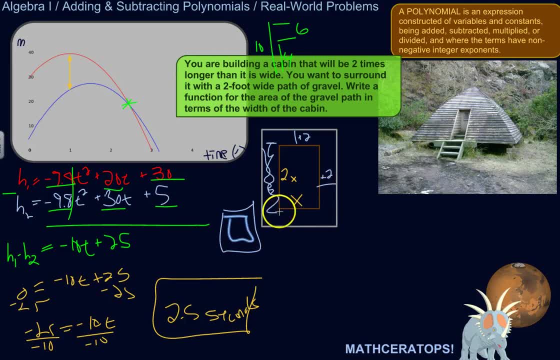 Okay, So what are the dimensions of the big rectangle? Well, if this is X, then- and I'm adding two feet, adding two feet- this dimension is X plus four. And then this dimension is: is two: X plus two plus two. 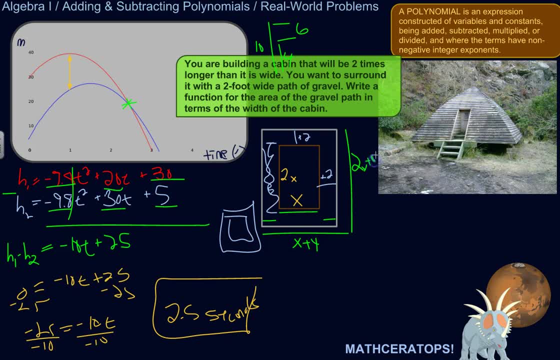 So this is two X plus four. So if I wanted to take the area of that rectangle I would just do X plus four Times two X plus four. That's the area of the big rectangle. So we can just FOIL this or distribute this out. 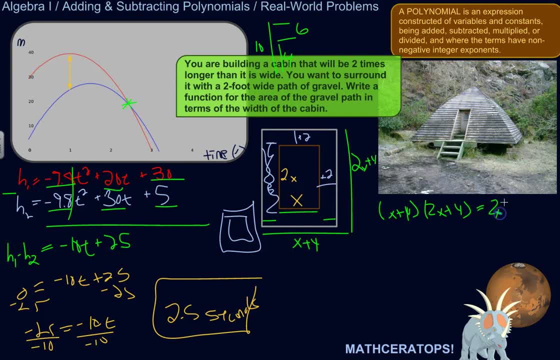 X times two, X is two. X squared X times four is four X. Four times two, X is eight. X. Four times four is sixteen. Let me write. let me write that Four times two, X squared Plus four X plus eight X. 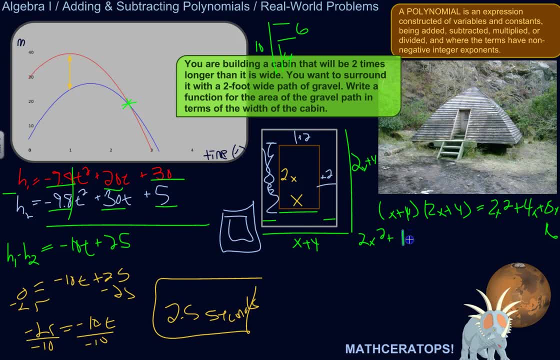 Let's combine those like terms as twelve, X plus sixteen, So that's the area of the, the large rectangle in terms of the width of the cabin: X. So we could, we could. basically, this would allow us to calculate the area and try different values of X. you know, if we're trying to design this cabin, 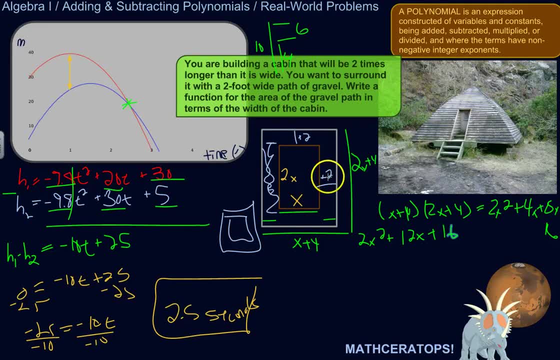 And we could see what happens to the area of the big rectangle. Okay, but we're going to subtract the area of the cabin because what we really want is the area of the gravel path. So the area of the cabin is two X times X. 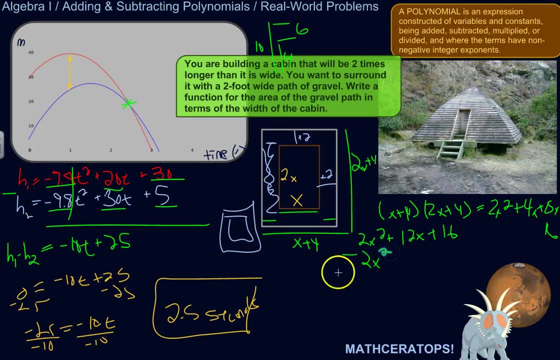 So that's two X squared. So if we subtract these two expressions, two X squared minus two X squared is gone. So all I'm left with is the area of the gravel path is twelve X plus sixteen There. So that gives us, so you know. back to the application. 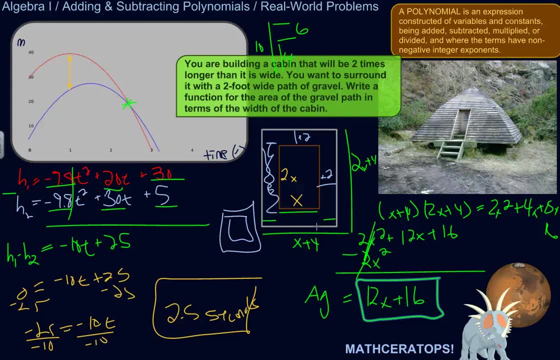 Maybe I'm designing my cabin and I'm like: well, maybe, maybe I want a cabin that's twelve feet wide. Would I have enough gravel To do a gravel path? Well, you know, twelve times twelve is hundred forty-four.